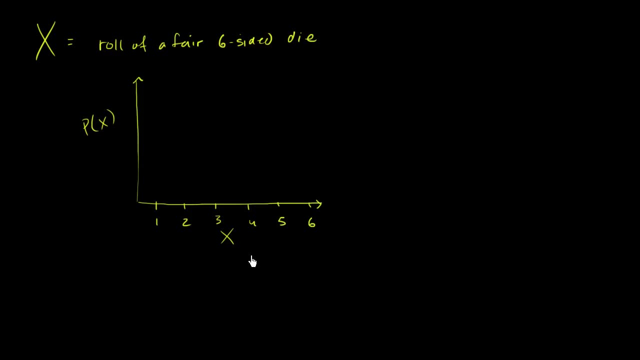 a 4. A 5 and a 6.. Now what's the probability of getting a 1 if you roll a fair, six-sided die? Well, it's 1 of 6 equally likely outcomes. So you have a 1 sixth probability. 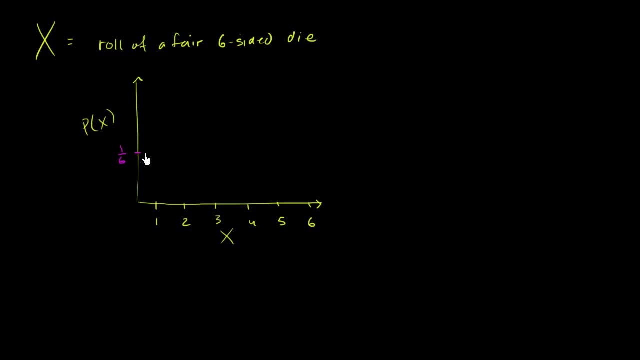 So it's 1 sixth. So that's the probability of getting a 1.. I'll draw this little bar chart here. So you have a 1 sixth probability of getting a 1.. Now what's the probability of getting a 2?? 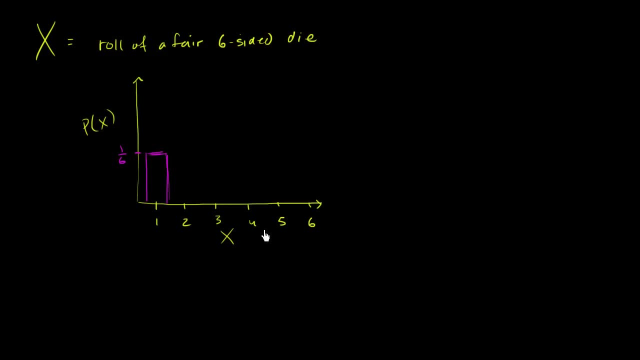 Well, once again it's 1 out of 6 equally likely outcomes, So it's once again 1 sixth. So I'll just draw it just like that. It is 1 sixth again, And same thing for 3.. 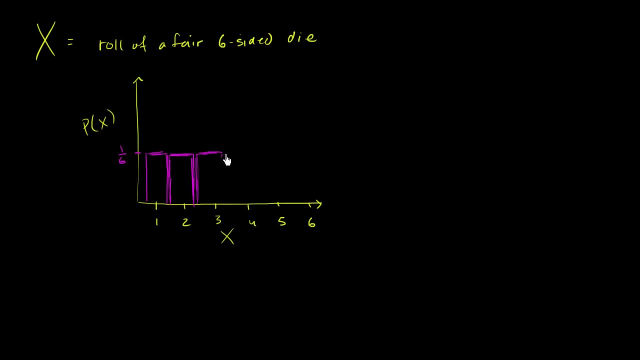 It's 1 of 6 equally possible outcomes, So there's a 1 sixth probability of getting a 3.. There's a 1 sixth probability of getting a 4.. There is a 1 sixth probability of getting a 5.. 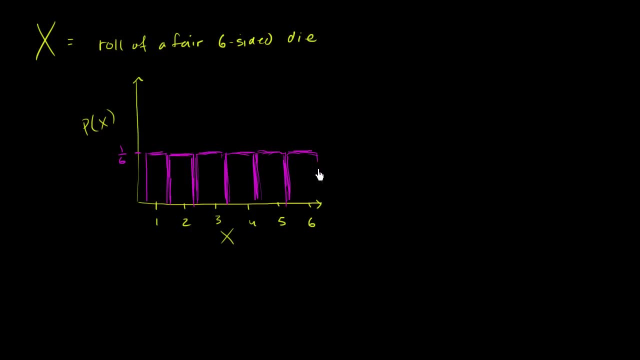 And there is a 1 sixth probability of getting a 6.. My little markers here got a little bit off center, But hopefully you get the general idea. So that's 5. And that is 6. Now the way that I've drawn it right here. 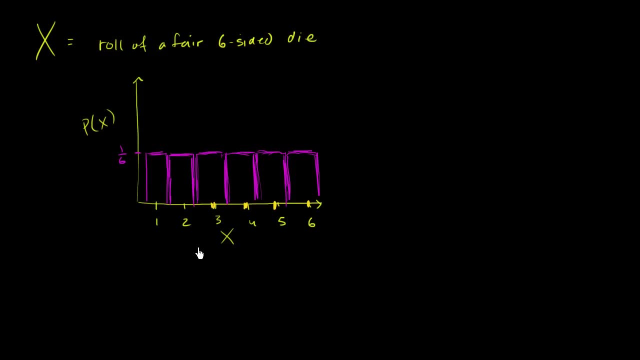 is this a legitimate probability distribution? Well, sure it is. You see that you have 6 equally likely outcomes. Each of them have a 1 sixth probability of occurring. The total, I guess you could say mass here if you say that there's 1 sixth in each of these buckets. 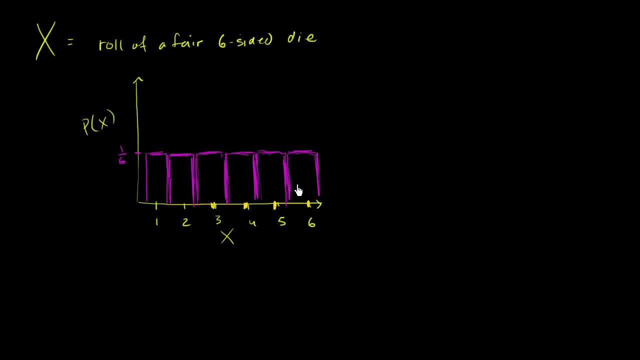 it's 6 times 1. sixth, It's 1.. It all adds up to 1, which makes sense. You have a 1 or 100% probability of getting 1 of these outcomes when you roll a fair 6-sided die. 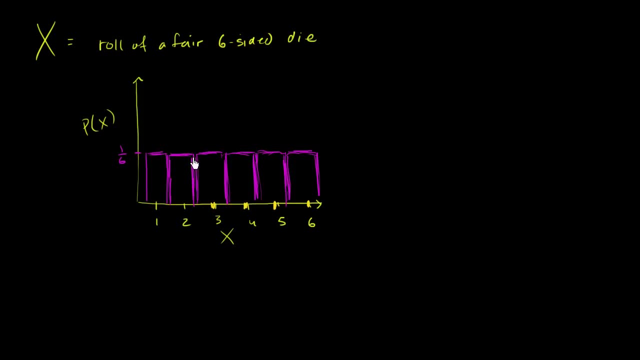 Now, when you have a probability distribution where every outcome is equally likely, like this- So notice: every outcome is equally likely. There's a word for it, just so you know it in the future if someone says that you're dealing with a uniform distribution. 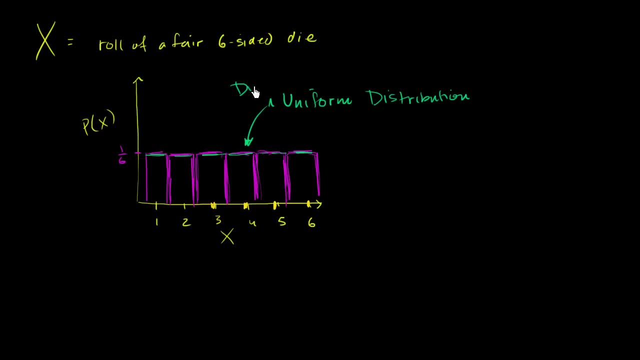 And you could have. You could have a discrete uniform distribution. That's what we have in this case, And in future videos we're also going to see continuous uniform distributions. Now my question to you. let's say that someone took one of these 6-sided die. 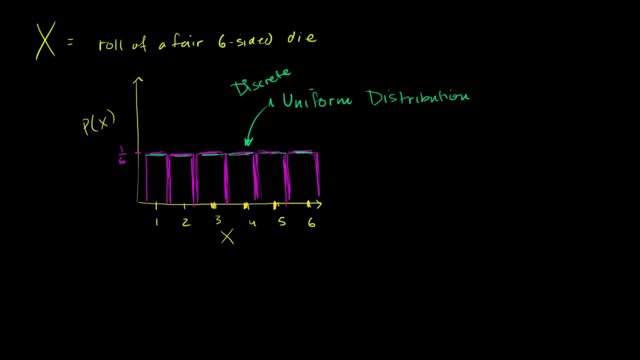 and erased one of the. so you have one side of the die that looks something like this where it has 2 dots on it And someone was able to erase it, So that side only has 1-sided. So now we're not going to deal with the role. 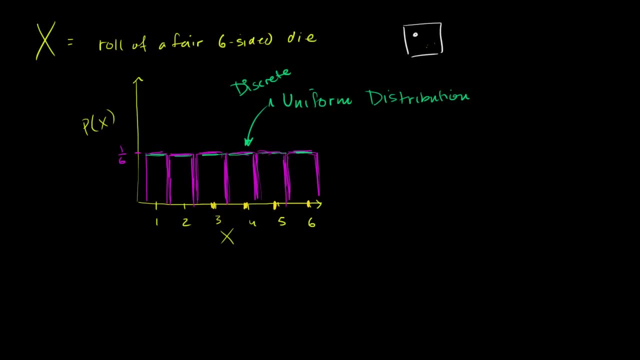 of a fair 6-sided die. It's still going to be a 6-sided die, but it's no longer fair anymore. It's no longer fair anymore. It's the 2-side replaced with another 1-side, Another 1.. 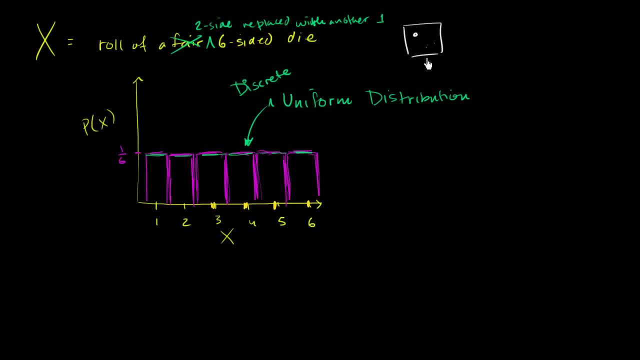 So you have 2 sides of the 6-sided die that are 1.. And then you have no side that has a 2 on it, And then the rest haven't been changed. You have a 3,, a 4,, a 5, and a 6 side. 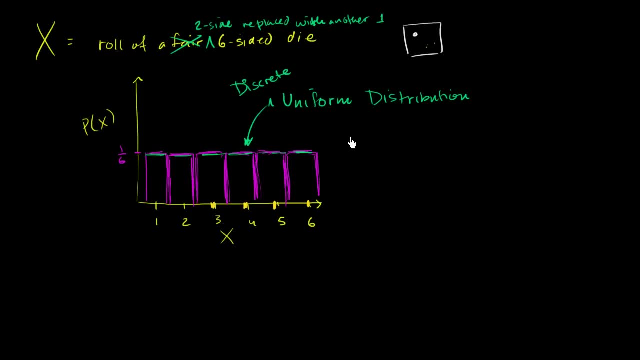 For this random variable. what would the probability distribution now look like? And I encourage you to draw it right now So you might guess that it will no longer be uniform. So let me remove this, just so we don't get confused, And let's think about it. 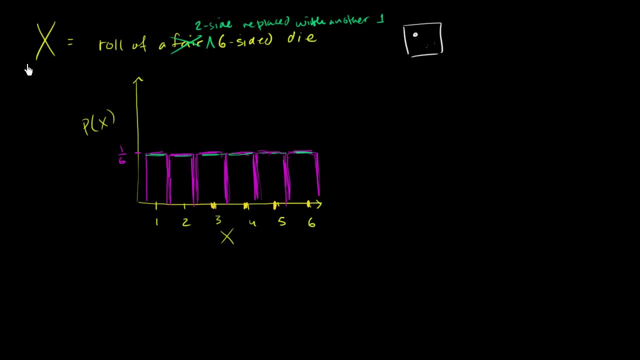 What's the probability for this new die that I get a 1?? Well, there's now two possible ways that I can get out a 1 out of a 6. So there's now a 2-6 probability that I get a 1.. 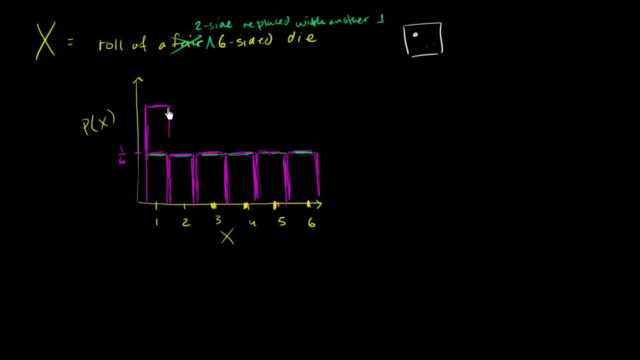 So let me draw that It's now a 2-6 probability that I get a 1.. So it looks like this all shaded in. So this right over here is 2-6.. Or I could write that as 1-third if I like. 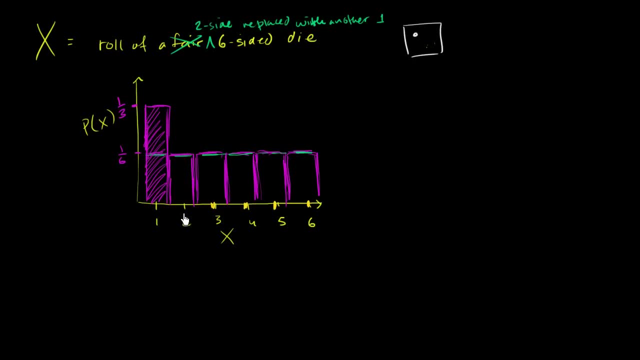 Now what's the probability of getting a 2?? Well, it's impossible for me to get a 2 now. There is no 2 on this die. I've removed the 2.. It's now a 1.. So there's nothing here. 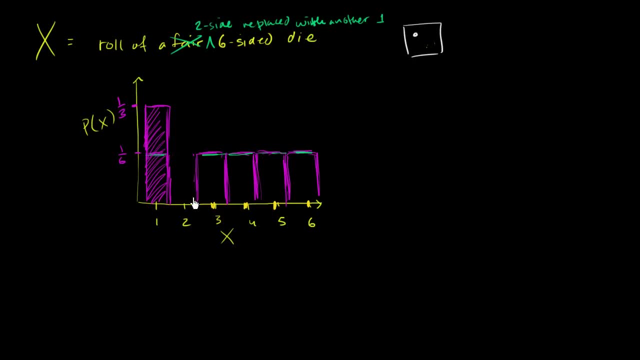 Let me delete all of this. There's nothing here. I have no probability. I cannot get a 2.. No face of this die has a 2.. Now what's the probability of getting a 3,, 4,, 5, or 6?? 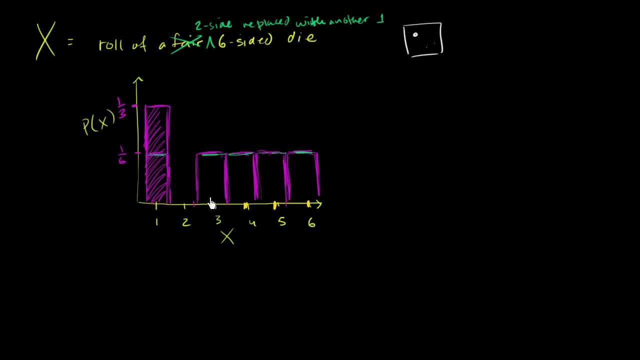 Well, those are unchanged. There's still one side that has a 3 out of six equally likely sides. So you have a 1-6 probability of a 3, a 4, a 5, or a 6.. So the rest stays unchanged.